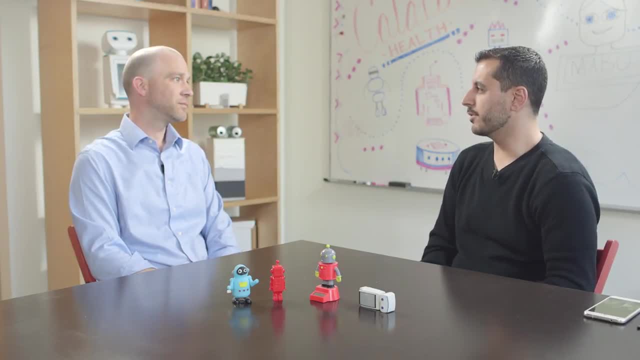 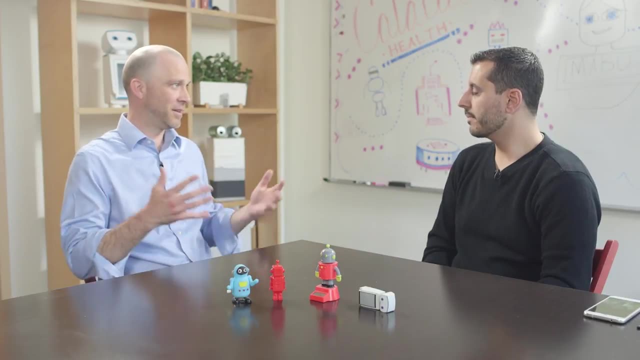 of interact with us and kind of work closely with us in building that bond between that technology. Well, I think it really depends on the application, right? Obviously, as humans, we've built technology for a very long time, right, It's something that we do And you know, you've. 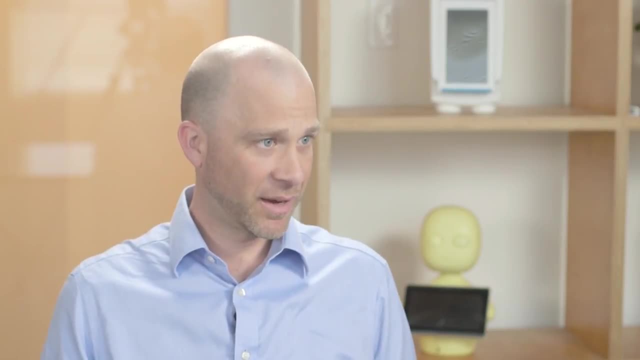 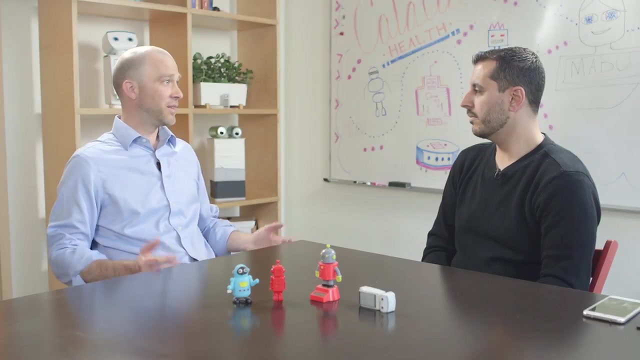 got a lot of technology Now that is getting more and more complex and doing things in the same physical spaces as us, right, And so part of that means stuff's moving around around us. Many of these take the form of robots or some other automation right, So the word robot is not necessarily 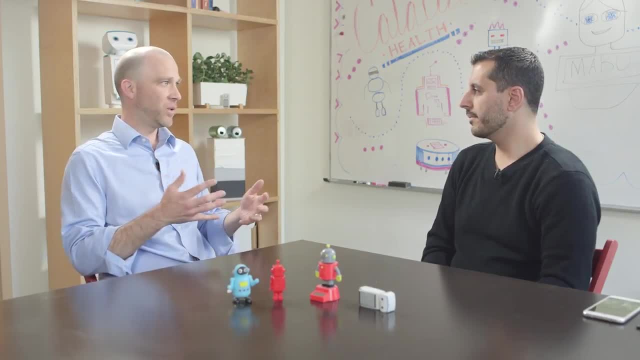 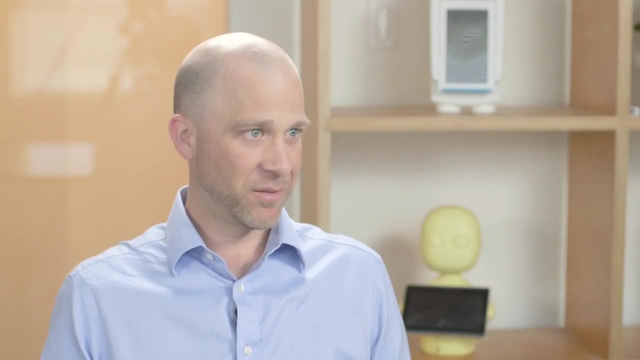 very clearly defined, right? So we could think about a lot of things that we interact with today or that we imagine that we're going to be interacting in the next few years, that are going to share space with us, And we need to know what that means. right, When this? 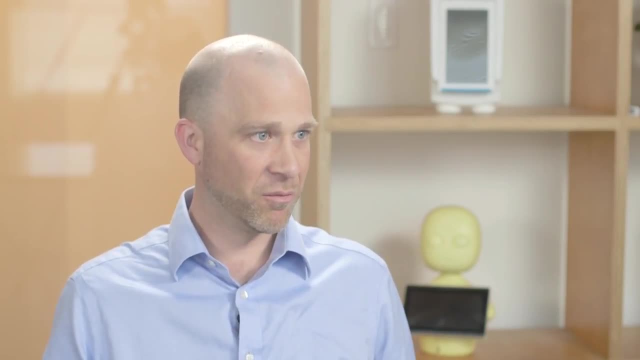 stuff is, you know, in our environments, in our offices, in our homes, you know, in our buildings, in other places where we're going to interact with it. understanding how that's going to work so that this technology is to our benefit and not our detriment, is very 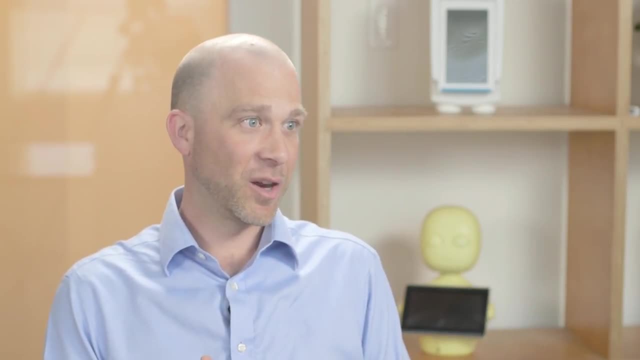 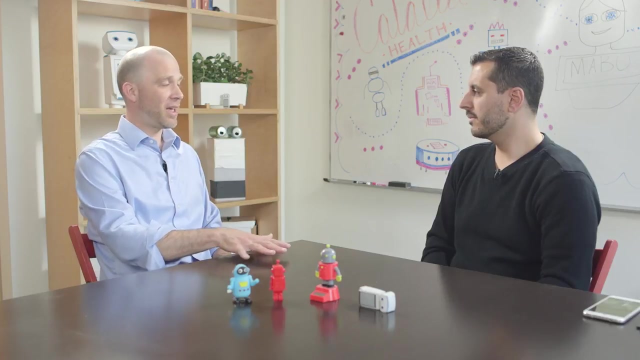 important right. So that's a very broad thing, very deliberately, in terms of you know how we think about this, the kinds of things that we're building. But I think that's a lot of what human-robot interaction as a field of study is about: right Understanding how. 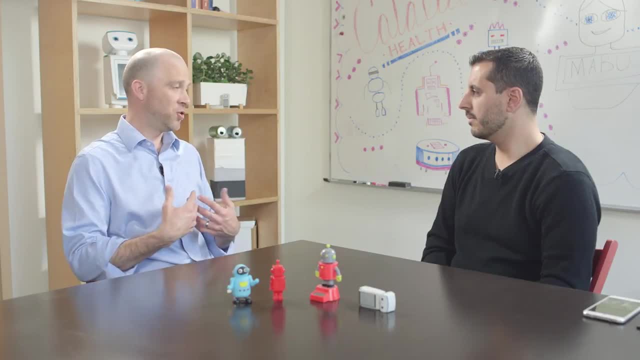 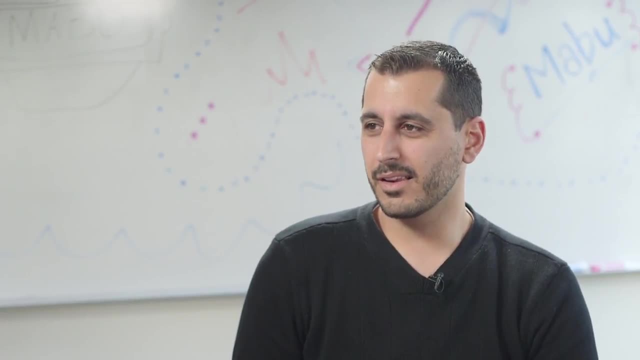 do we solve these problems in a way that benefit us as humans in terms of using this technology? What kind of studies are you aware of that have kind of taken place- Yeah, That have taken place in this area that really kind of started to drive this movement, that. 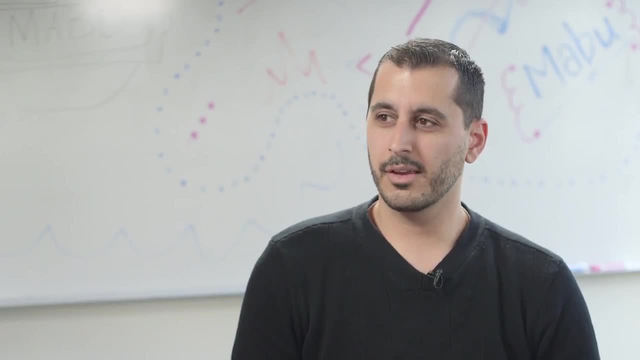 were kind of like a focal point that people started saying, hey, we really need to kind of, you know, focus a lot more on this aspect of how people interface with machines and not necessarily just that the machine is here and it's going to do a job and we really don't. 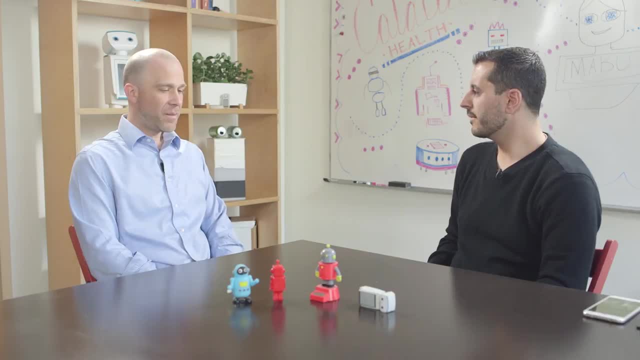 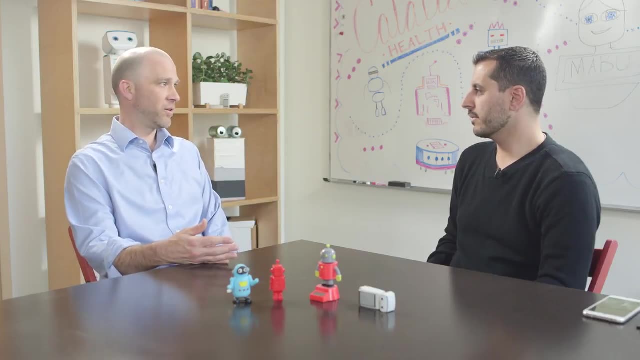 care about how it ties in socially Right. So I mean there are thousands of studies in human-robot interaction that have been done over the last two decades And that really builds on the field of human-computer interaction, where you've got many, many more studies going back for, you know, a few years. 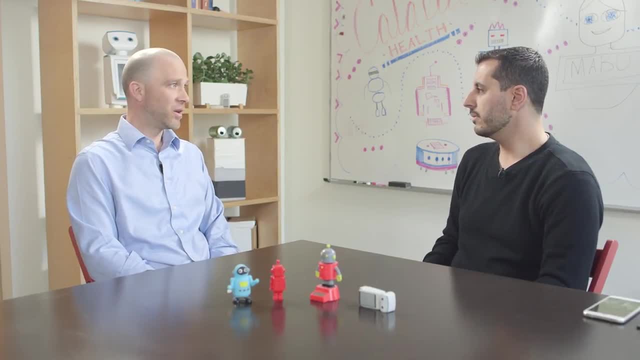 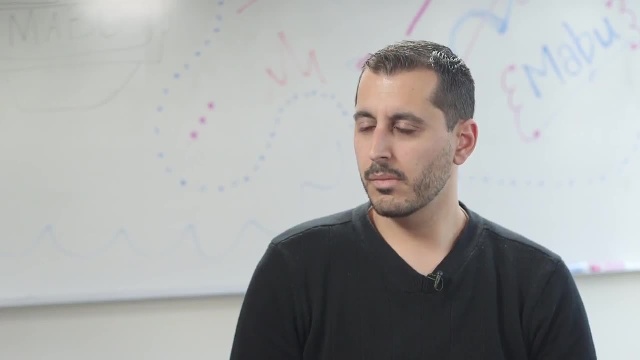 going back for about a half a century now, probably even longer. So you know it's a field that people have thought about for a long time And you know so a lot of different aspects to these studies. Some of them are, you know, very broad and trying to understand. 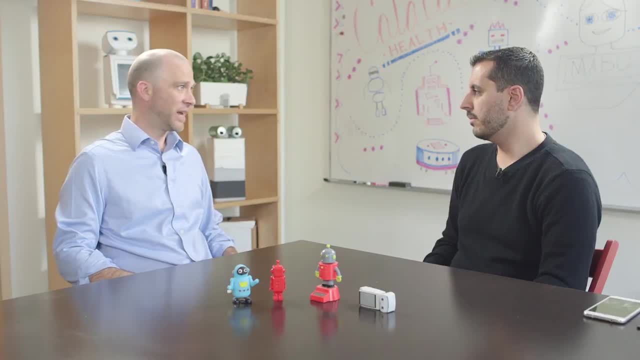 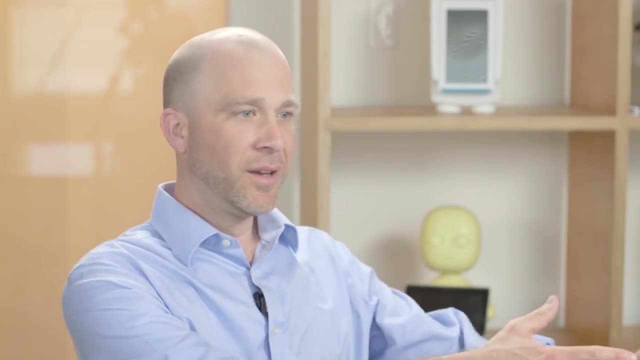 you know, you put robots into a particular environment, how do people interact or react? Some of them are very specific, right? So, getting down to some of the details, you know, if we have a mobile robot, say, that can move around, how close can it come to you and you're? 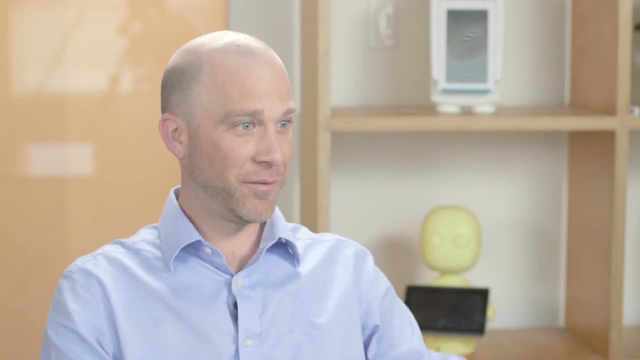 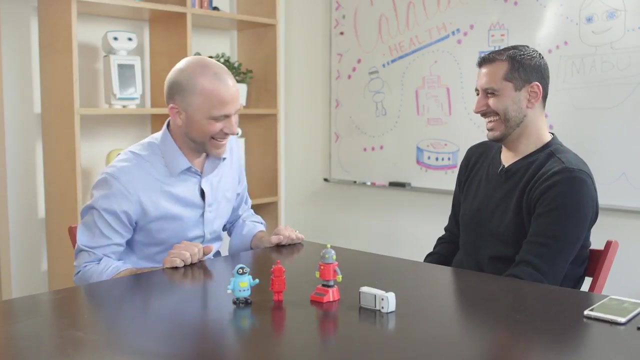 still comfortable, right? So very similar to, you know, interpersonal space. We're a few feet apart right now, right? This would be a bit different if we were like right up close to next to one another, right? So you start to feel awkward when I get into. 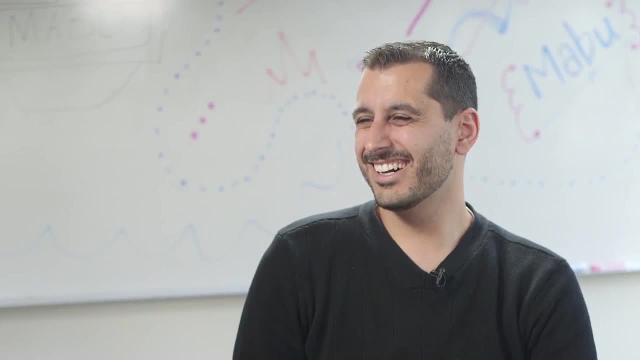 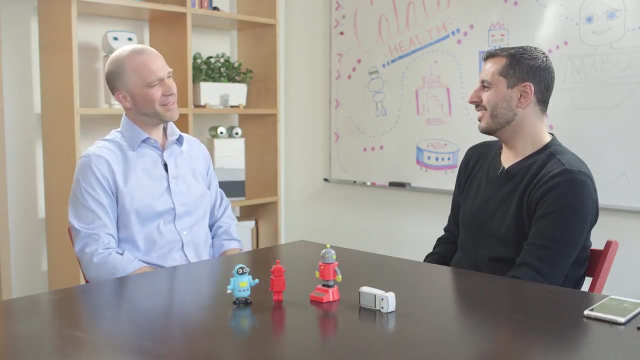 your face. Same kind of thing with robots, right? Is it the same as with us, right? Is you know? six inches too close with a robot, Definitely is. if you know we were talking six inches apart, Three feet. This feels about right, Is it the same with a robot? So you've. 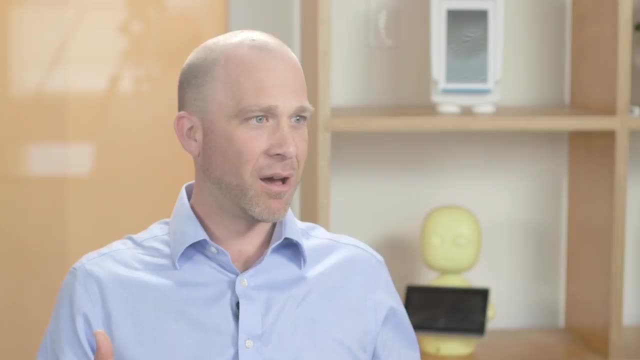 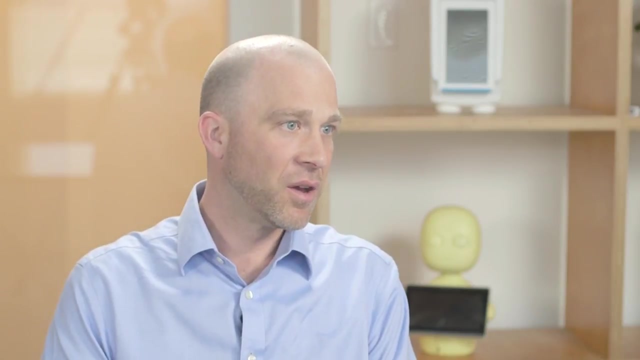 got a whole range of things and you can imagine all different aspects of interpersonal interaction right with other people. How do we apply those in the world of technology, specifically in the world of robotics? So there's this whole body of literature again looking at. 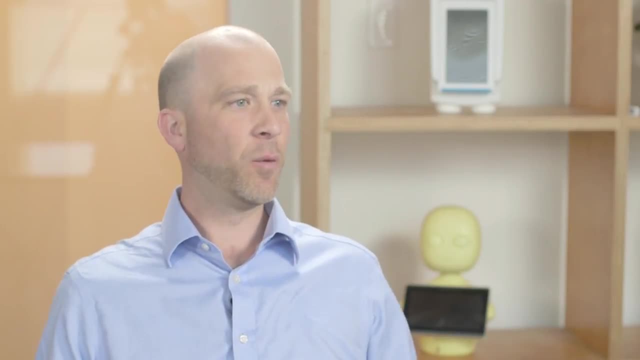 the very broad things: right Robots in particular situations, or how do they help us in education or healthcare or entertainment, to the very specific. you know if a robot does this particular action or says this thing, or, you know, makes this sound or right these very specific 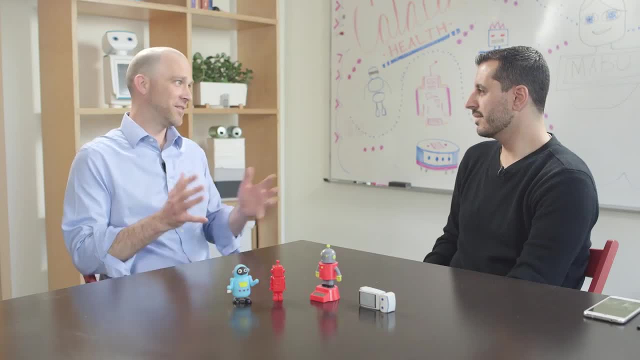 pieces. there are a lot of studies around that as well. Now doesn't mean that the field is done right. There's so much more that we have to understand for a couple of reasons. One is: you know, there are perhaps an infinite number of those types of questions that we can answer right. 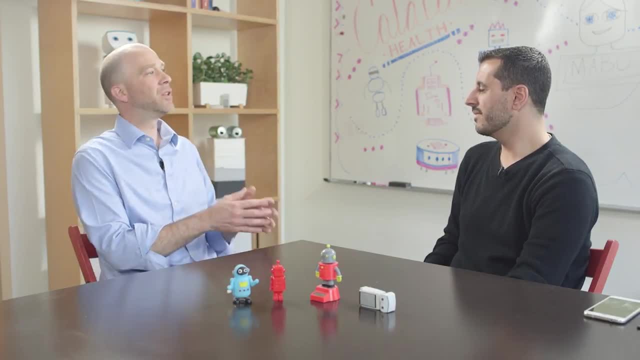 We can keep thinking of new ones, but also the technology is evolving, right? If we look at what an interactive robot or a social robot is today versus what it was five years ago or ten years ago or twenty years ago, the technology is very different. Its capabilities. 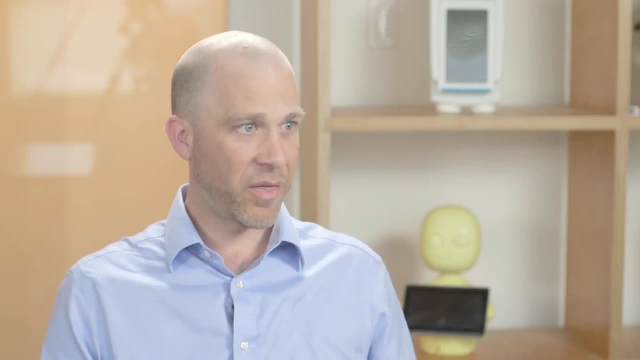 are different And as we continue to develop new things, whether that be the technology or the use cases for it, then we need to keep exploring these interactions. And again going back to how do we make this technology in a way that benefits us as people and the user? 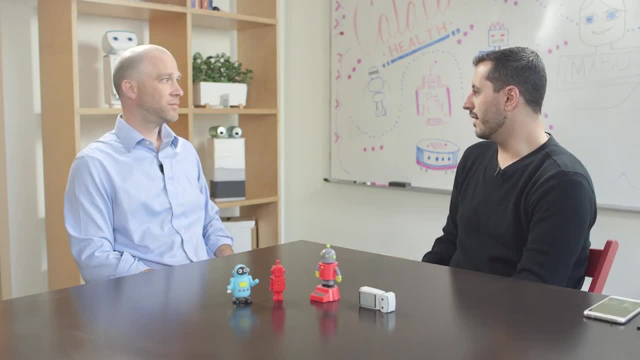 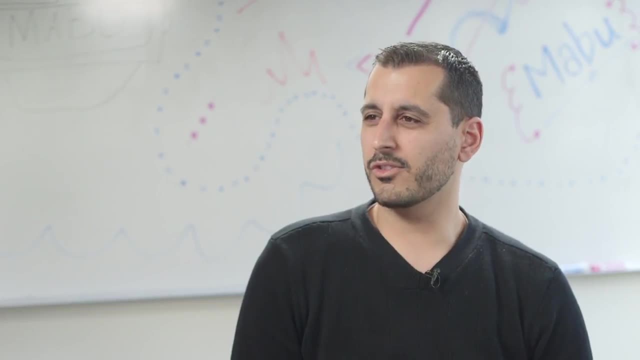 of it. So, looking at some of the studies that have been done, right from a psychological standpoint, how would you conduct one of those types of studies Like what would you find that would be useful information? So, for instance, I know you got close to my face a few seconds- 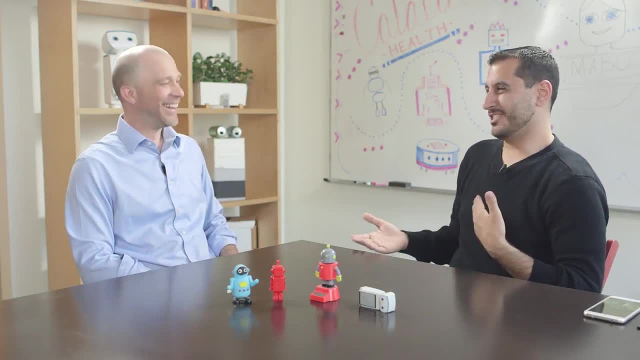 ago and were like: does this make you uncomfortable? Great way to do it right. And you know, for some people it does. For me personally. I have a very small personal bubble, so it doesn't really bother me a whole lot. 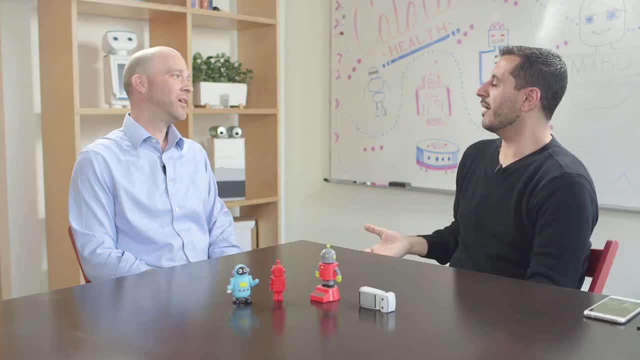 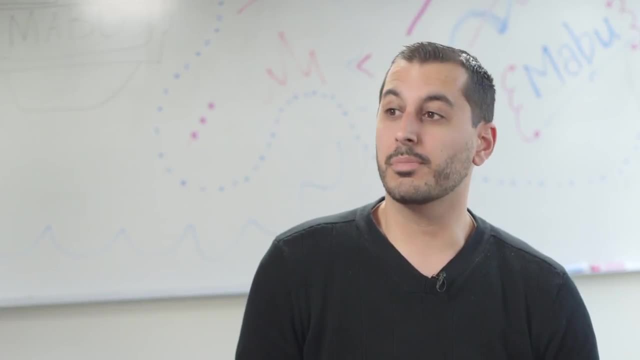 I know I saw that look So, but in those situations, though, right, there's generally a distance that people typically like to hold right. A lot of it's cultural, some of it's social right, Some of it's just personal, But how? 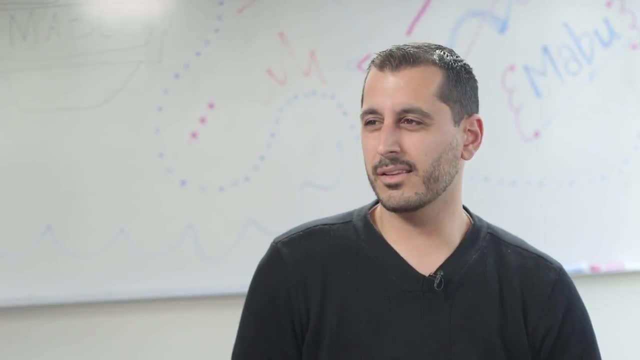 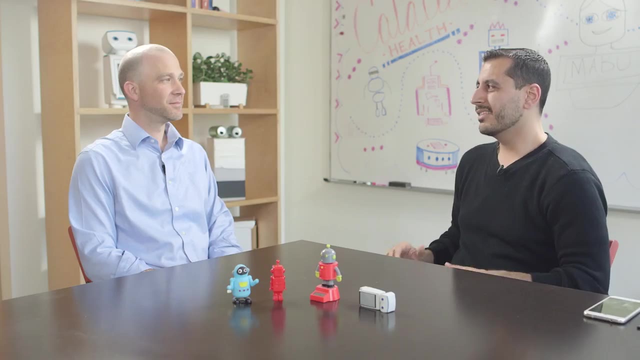 would you go about setting up one of these studies? What kind of studies like these are typically conducted when you're trying to do some sort of research for human-robot interaction, where you're trying to say, well, a robot four feet away is okay, a robot two feet away? 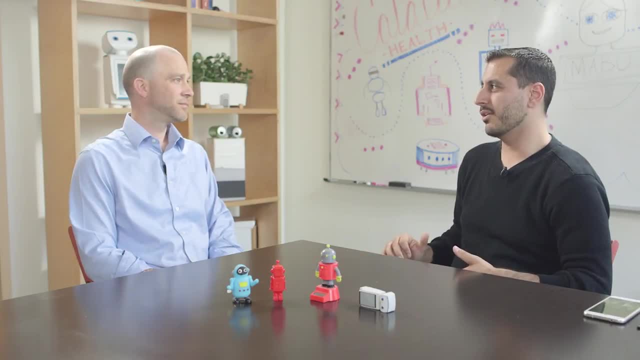 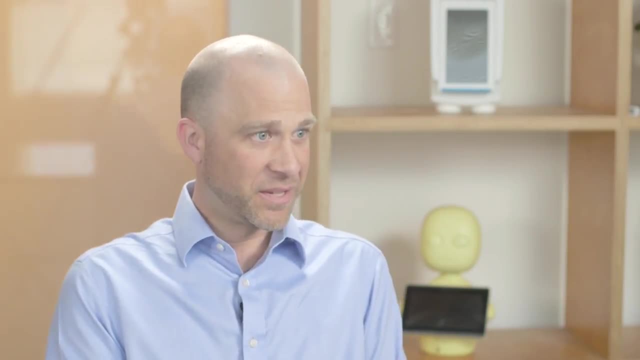 not so much. Or a robot that's two feet away, that's six feet tall, I really don't like, But if it's only a half a foot tall it doesn't really bother me a whole lot, Sure. So I mean, some of those questions are very specific, right, And you can imagine. 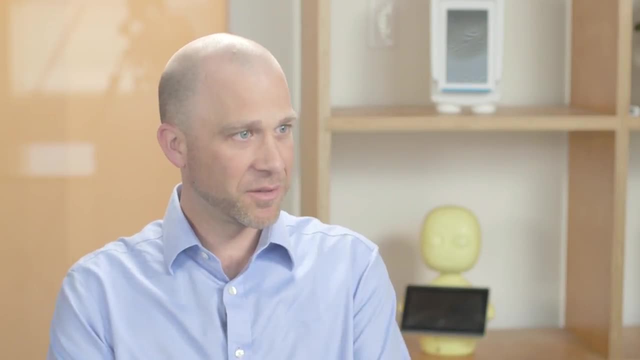 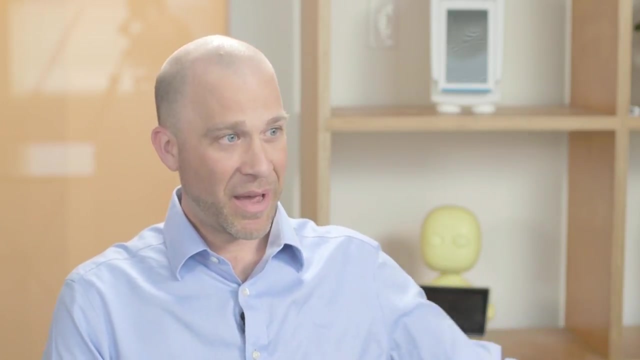 how to design a study And you know any particular study needs a design That's appropriate for it. But as a rule of thumb, again I'd go back to psychology. So when I was starting off doing my master's degree at the MIT Media Lab 16 years ago, 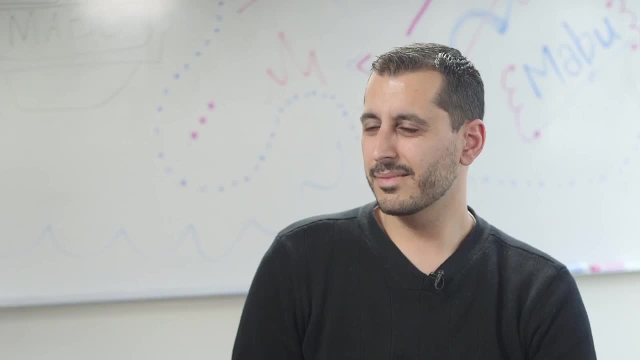 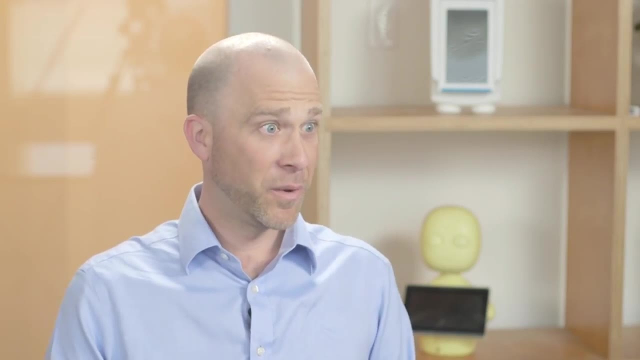 one of my mentors was the late Cliff Nass at Stanford And Cliff semi-jokingly would talk about his research methodology as this. He'd say: so Cliff was an expert in human-computer interaction right Later went on to do some work in robotics. But he would say: you know? 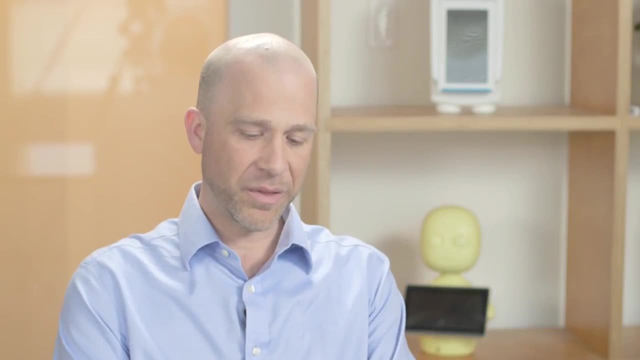 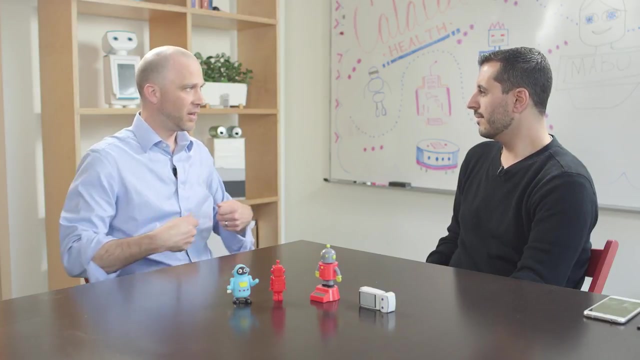 go into the psychology section of the library, right, And I'd find a paper with a great study about two people interacting with one another. And I would take one of those people, cross it out, put computer and steal it right And 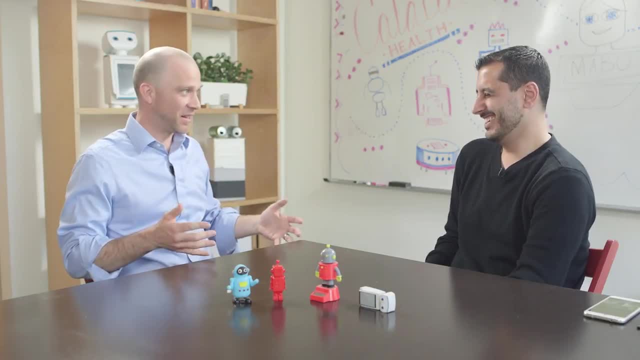 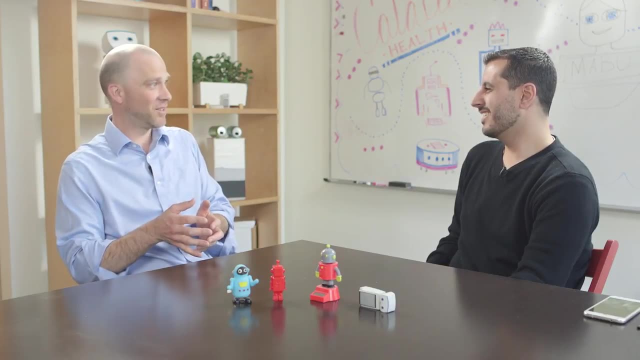 so you know, he ended up publishing- I don't know, possibly hundreds of studies, right, A lot of different studies of human-computer interaction. Now, he was very clever then about how he translated those into the world of people interacting with technology. But 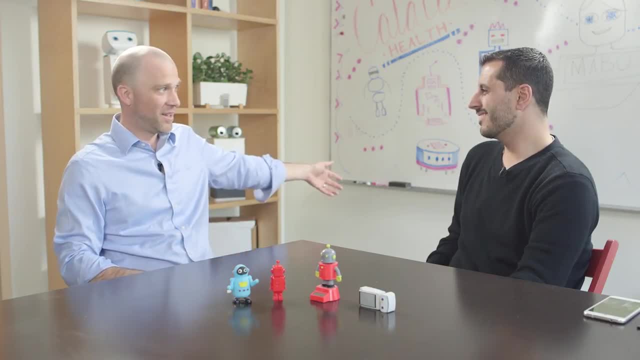 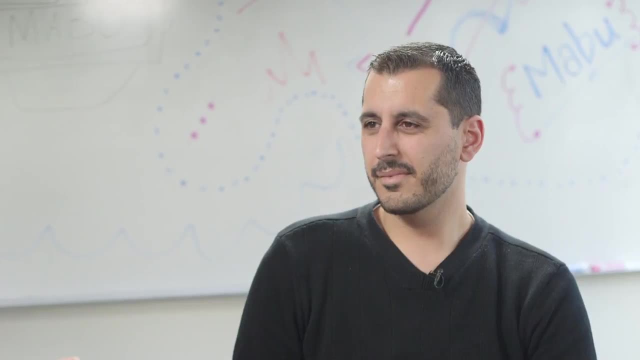 in general, that's a great technique. So some of those early studies that I was doing, you know, more than a decade and a half ago, Cliff and I designed together right, Really using that kind of methodology. Okay, if there's this kind of a problem that you want to solve or this kind of a thing, 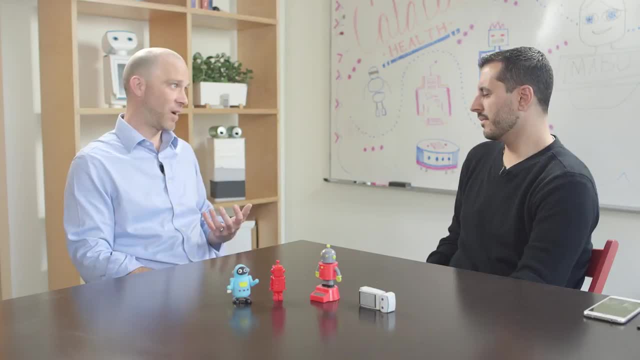 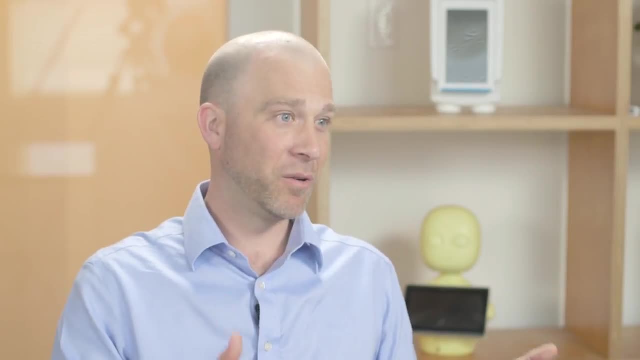 you want to learn again. there's a great precedent in how do we, as people, interact with one another. Let's go borrow from that right. Let's learn what we've already used in, you know, academic or research settings to understand how people are interacting with. 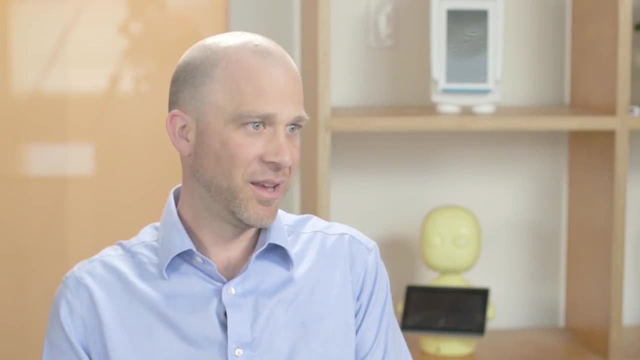 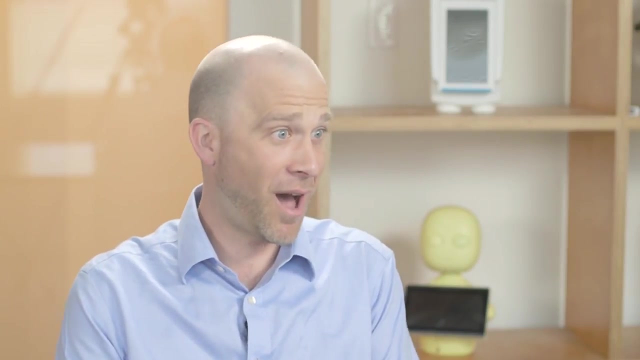 one another and understand how we apply that with technology, And so it's a great way to think about that right Again. what we're building in terms of the technology is very new. What we're creating in terms of the interactions is not right. We really want to leverage what